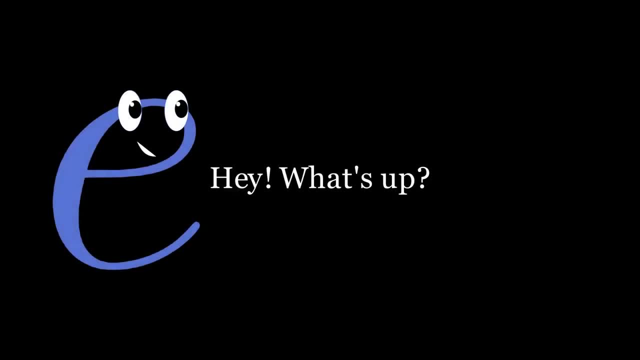 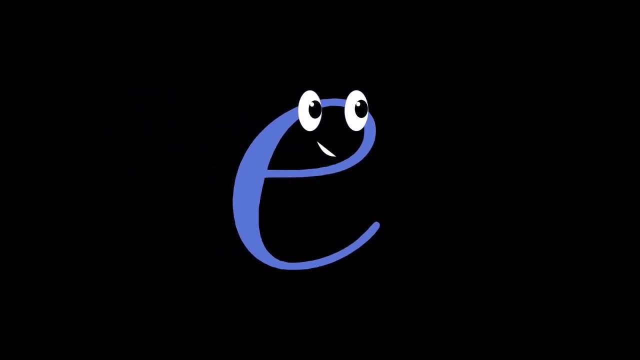 Hi mates, how are you doing? Today we are going to prove a very interesting and important theorem among many branches of mathematics, And that is the Cantor's theorem. First of all, let's try to understand what our theorem actually says. Take any set A. 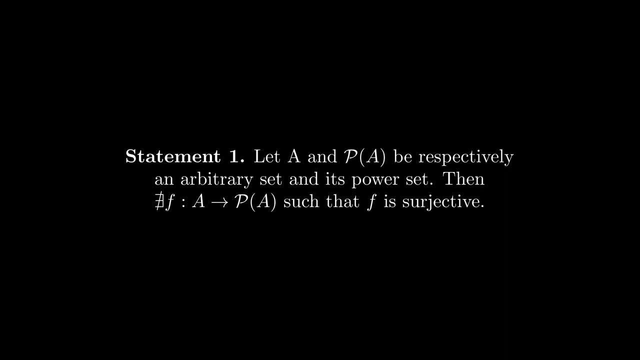 and its power set, Then our result implies that no function from A to its power set is subjective. That is, you can choose any function f that goes from A to its power set. This function f is never going to be subjective because there's always going to be some element. 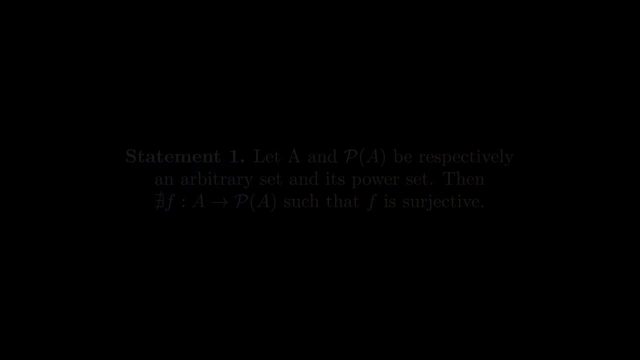 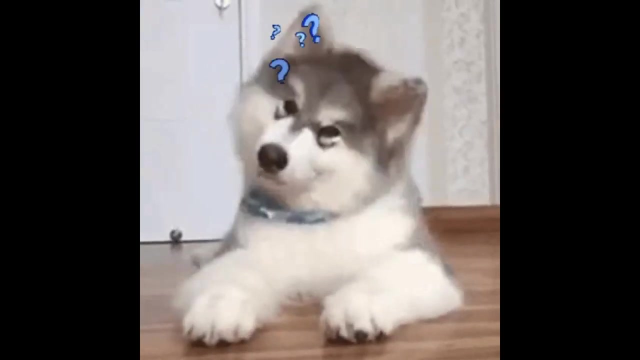 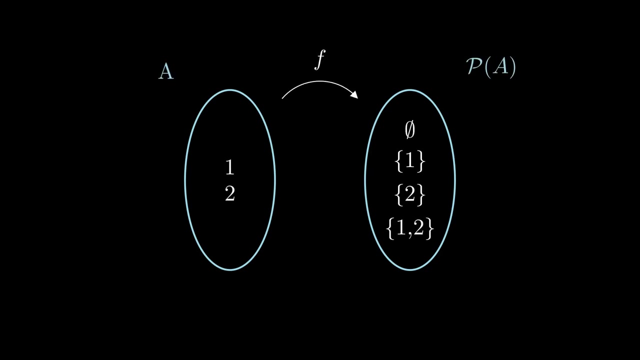 in the power set of A that is not in the range of f. I know it might sound a little bit confusing, but it is actually quite simple. So let's take a look at some examples and sketch out some stuff. So suppose you have a set A that has, I don't know, two elements, one and two. 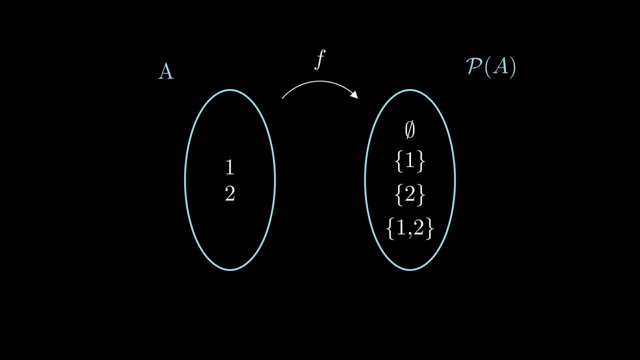 Then take the power set of this set. If you try to draw a function from A to the power set of A, you are always going to fail to make your functions subjective. For instance, consider the function f that assigns to each element x the subset of A that 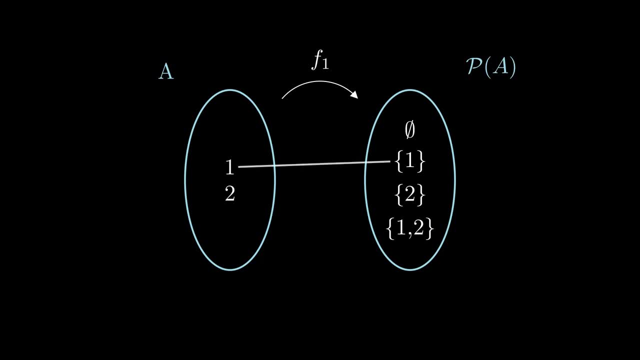 only contains x. If we plug the number one into this function, our output will be the set that only contains the number one and the same for the number two. Do you see what happens here? There are elements in our codomain that are: 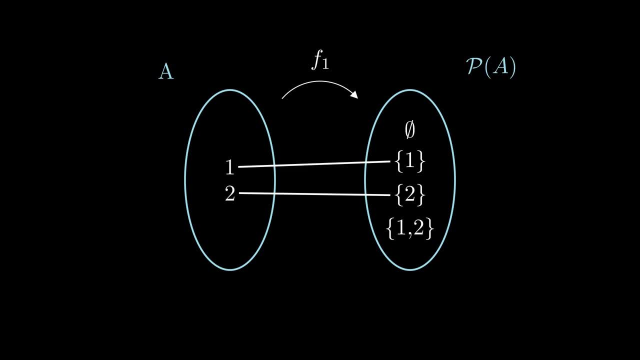 not in our relation, f1, and hence f1 cannot be subjective. We could also choose an f2 that does the exact opposite of what f1 does. I mean for the number 1, let's assign it a subset of a that does not contain it, Same for 2.. Similarly to our form example, f2 isn't subjective either. 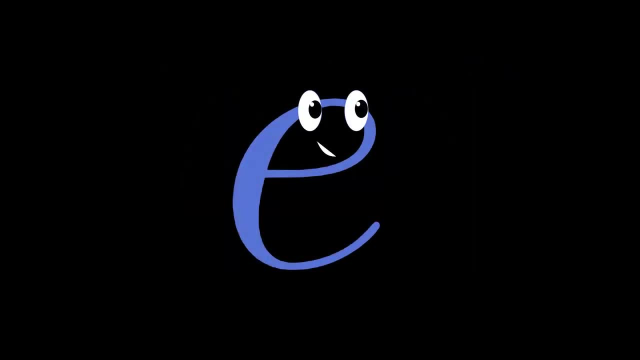 Well, for any set, a that is finite, it is quite intuitive to notice that there can't be a subjection from a to its power set, since a will always have fewer elements. More precisely, the power set of a will always have two to the n elements, n being the number of elements of a. 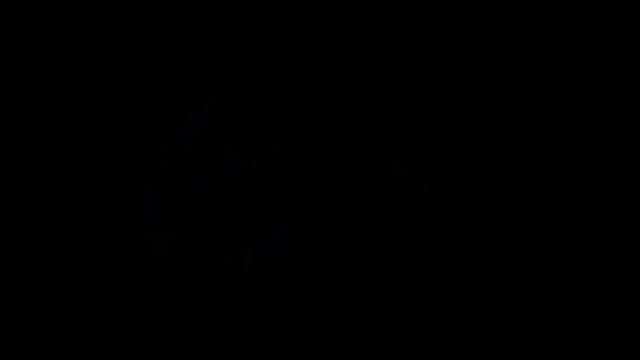 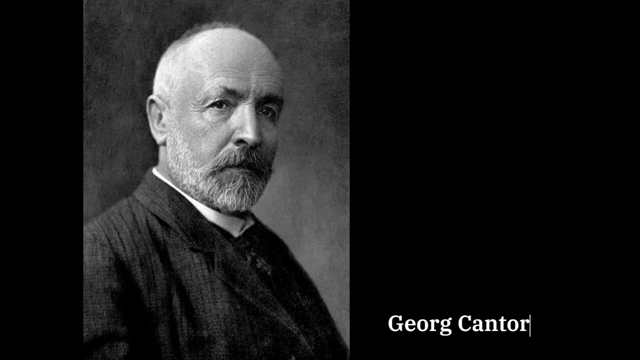 All right, but what if a is infinite? What Cantor was able to prove is that, even if a is not finite, the cardinality of a power set of a, or the number of elements of it, is always going to be strictly greater than that of a. 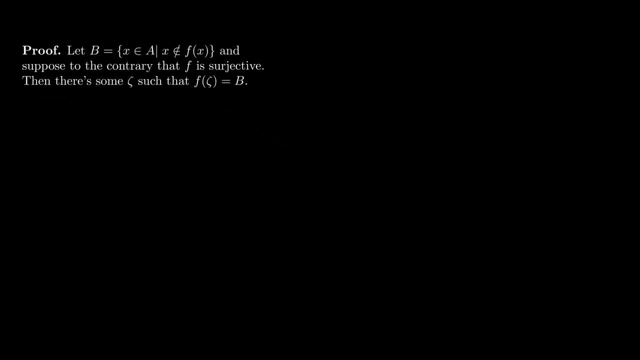 And to do this, we're going to need a set of elements of a. And to do this, we're going to need a set of elements of a. To do that, we first assume, to the contrary, that there is a subjection f through a to its power set. 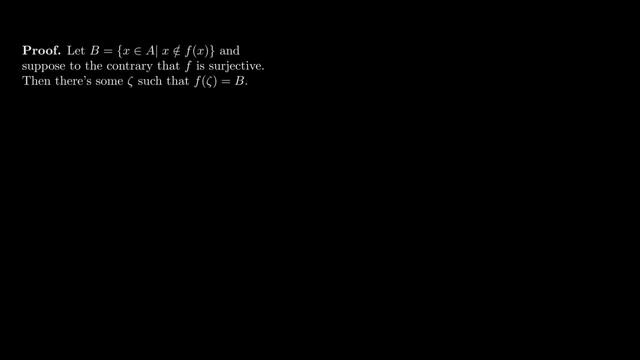 Then we define a set b such that if x is an element of b, then x is not an element of its own image through f. That is, if we plug x into our function f, our output will be a set that might or might not contain x. If it doesn't contain x, we add x to b, otherwise we just ignore it. 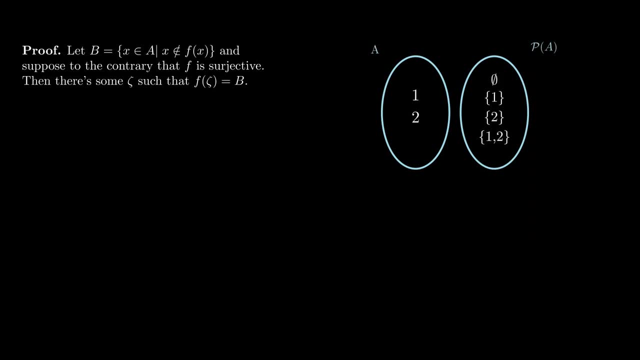 Yeah, we can totally do that. In fact, we did this with our previous function, f2.. b in that case would be the whole range of f2, and if we took f1, for instance, our set b will be an empty set. Anyway, here it's important to notice that b is also a subset of a, since it only contains the 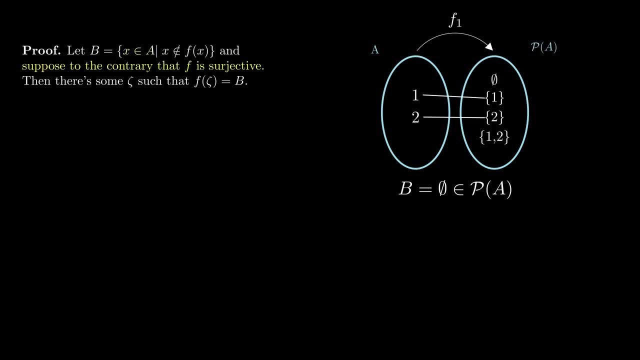 element x, but are also elements of a. Since we assumed that f is a subjection, it follows from its definition that there is some element in a such that f of this element is our set b. Since we assumed that f is a subjection, it follows from its definition that there is some element in a such that f of this element is our set b. 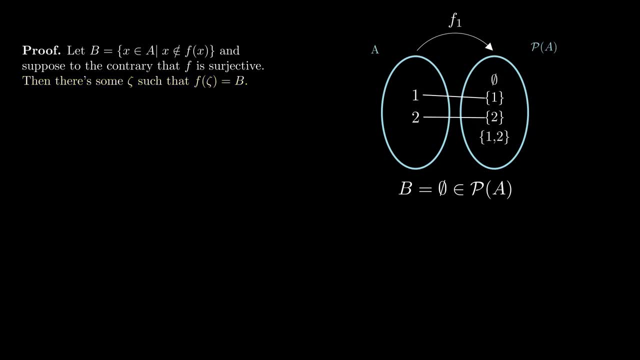 Since we assumed that f is a subjection, it follows from its definition that there is some element in a such that f of this element is our set b, Since b is a subset of a and we can call this element zeta. If zeta is an element of b, then according to the definition of the set b, 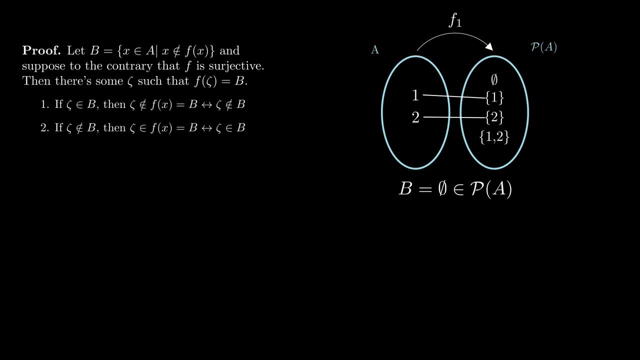 zeta is not in its own image through f, but its image is b and for this case we've just assumed that it is an element of b. thus we get a contradiction. And if zeta is not an element of b, still following the definition of b, zeta is in its own image through f, but f of zeta. 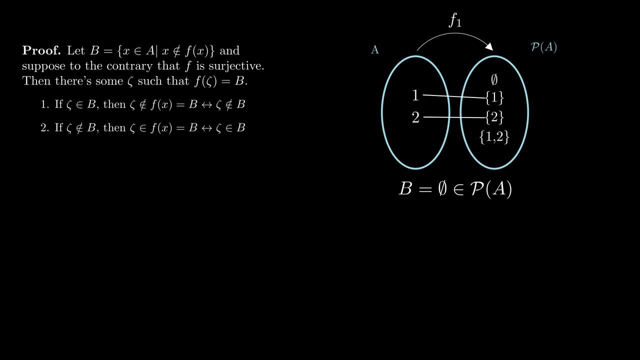 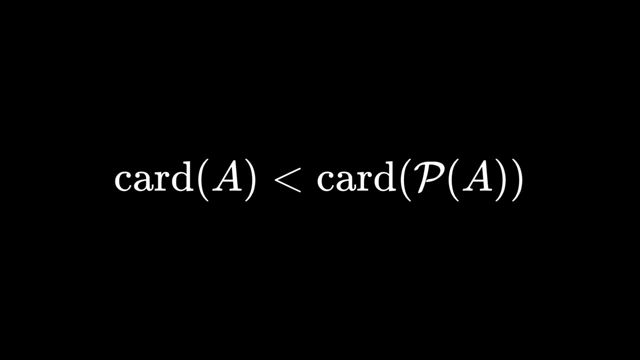 is b, that is, zeta should be in the set b. again we get a contradiction. Since assuming there is an f that is subjective brought us a contradiction, we must include whether it can't be such an f. Take our f1 again. This function is always going to be injective.